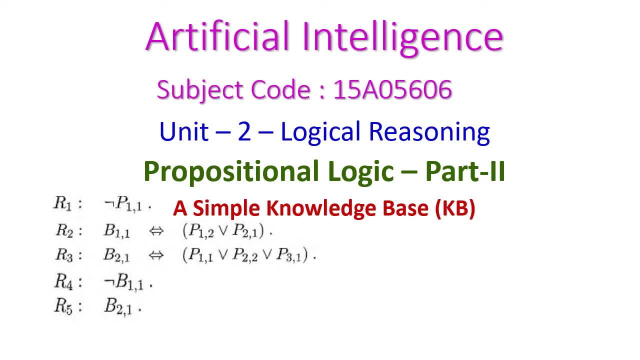 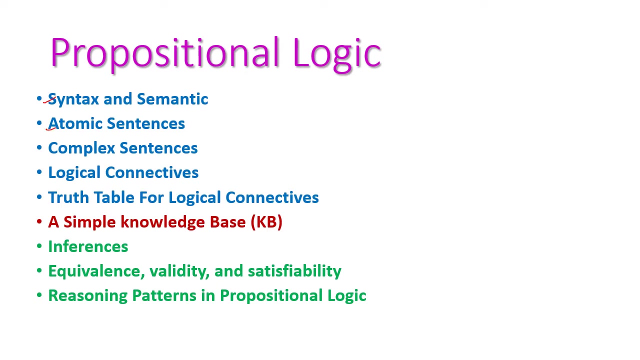 Hello friends, welcome to today's artificial intelligence class, and in this class we will see the second part of propositional logic, and here we are going to construct a simple knowledge base, that is, KB, from this second unit, logical reasoning. In the last video we have seen the syntax and semantics of propositional logic, atomic and complex sentences of propositional logic, and after that we have seen the logical connectives, that is, the five logical connectives which will help to create a complex sentences. 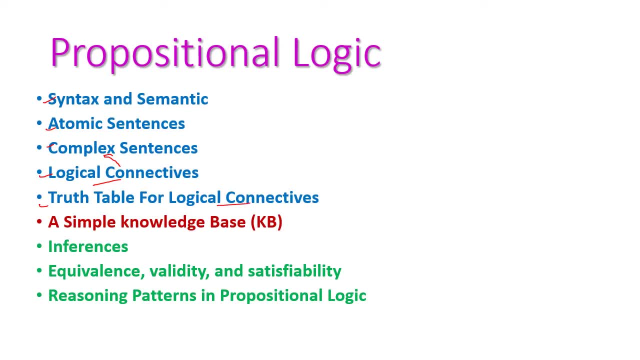 After that we have seen the truth table for those logical connectives And in this class we will see the simple knowledge base, that is, we are going to create A simple knowledge base. In the next class we are going to see the inferences, equivalence, validity and satisfiability. after that reasoning patterns in propositional logic. 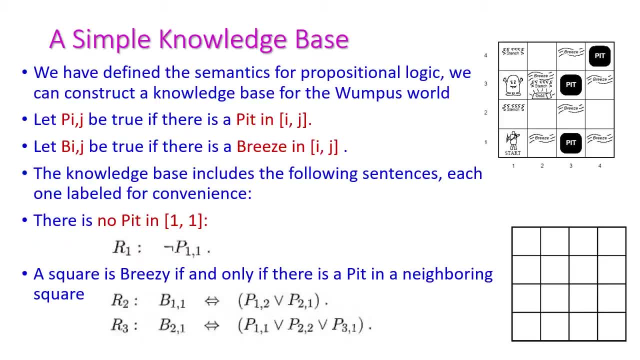 So in the next video we will see all these things right. A simple knowledge base, right. So for creating this simple knowledge base, we will take this Wampus world example, because already we have seen this Wampus world example in our previous video, Isn't it? 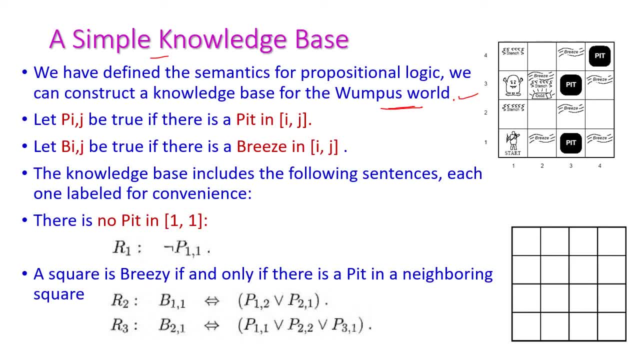 So already we know what are the concept in the Wampus world. So for creating a simple knowledge base, let us take this particular one P of I J Here. P is the pit and I, J is position in this Wampus world. Okay, 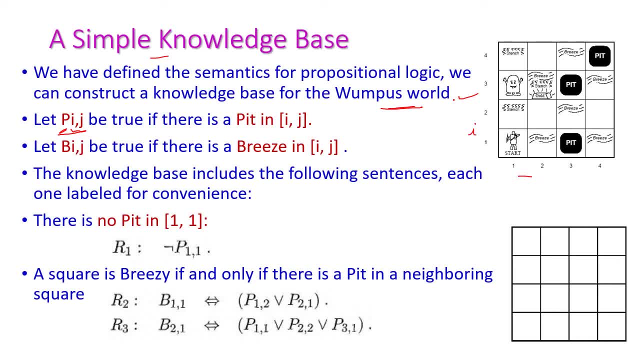 I throw. This is I and this is J. Okay, I J Right. If P of I J is true, If, and only If, there is a pit in I J. Okay, The meaning of P of I J means there is a pit in I J. 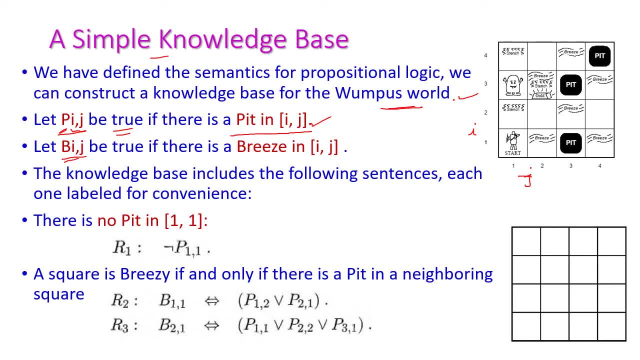 And next B of I J. B means breeze, Isn't it So? B of I J, If B of I J be true, If there is a breeze in I J, Right, Okay, So by using this only. 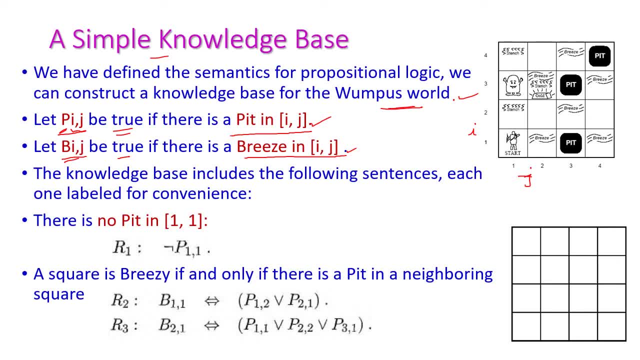 We are going to Construct our knowledge base. Okay, So the knowledge base includes the following sentences, Each one labeled for our convenience. Okay, So the first sentence is: This is the first one. There is no pit in 1, 1.. 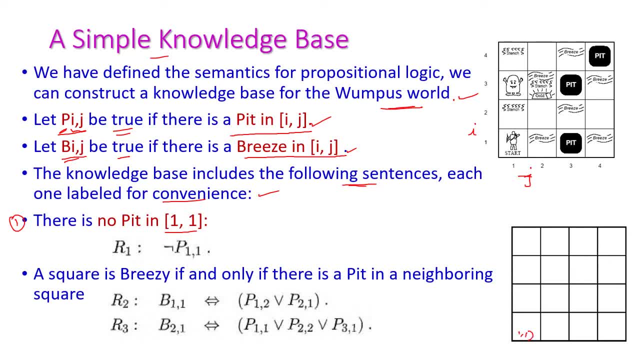 So in this, 1, 1.. 1, 1. No pit, Okay. No pit means negation of pit of 1, 1.. This is the first one, First sentence, Okay. And when come to second sentence, 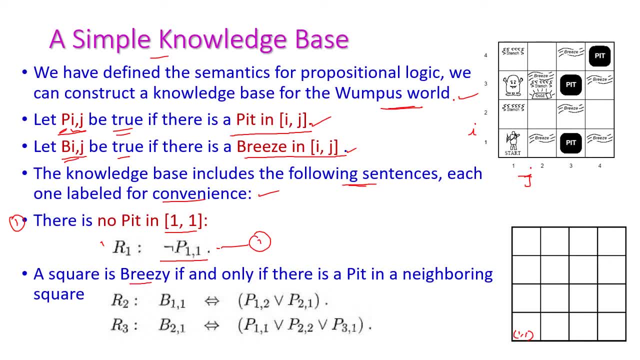 A square is breezy If, and only if, There is a pit in a neighboring square. Okay, From our example we can see If there is a pit in 1 square means All the neighboring squares Will be Breezy. 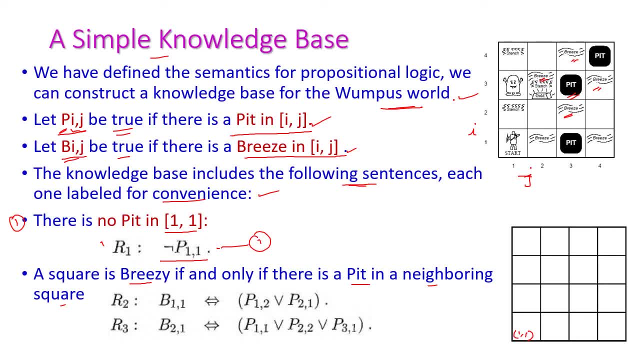 Okay, so r2, that is the sentence to b of 1 comma 1. so here, suppose b is there, then pit may be in 1 comma 2, 2 comma 1, 1 comma 2 and 2 comma 1, isn't it, if a pit is either in? 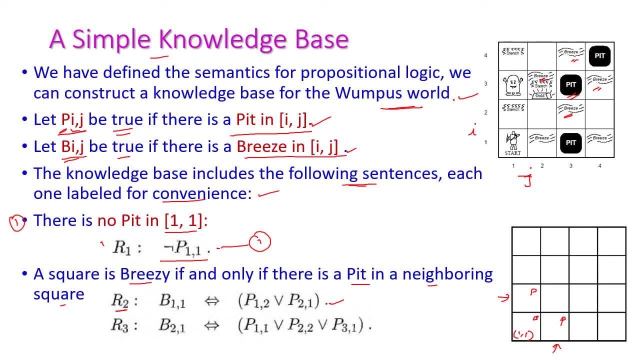 this square or in this square. so we have to use this r symbol, that is disjunctive symbol, right? okay, and this is the second one. and when come to third one, okay, if b is in 2 comma 1, suppose, if b is here, if the position is b is here, then p. what is the place of pit? 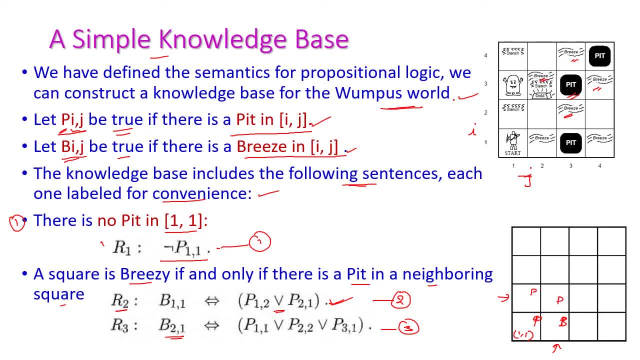 pit may be here. pit may be here. pit may be here. okay. pit may be in 1 comma 1. pit may be in 2 comma 2. pit may be in 3 comma 1, right. so this is the third sentence, then all the neighboring. 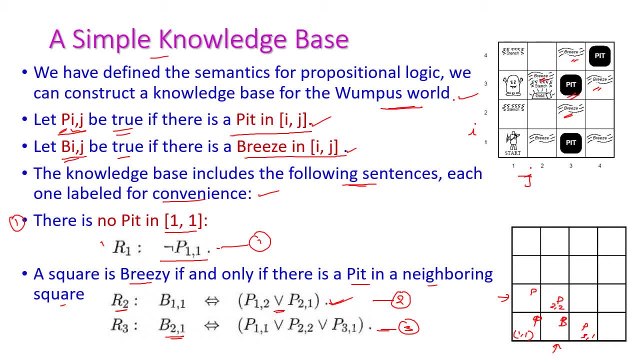 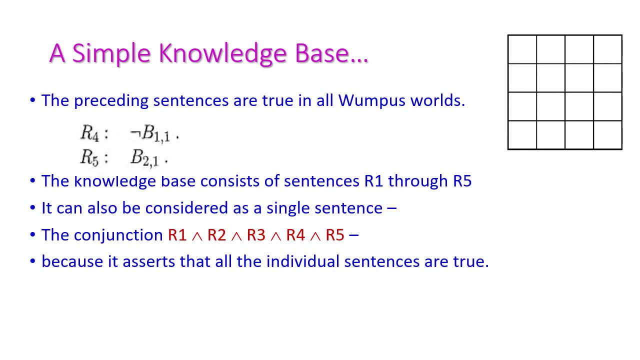 squares. any one of the neighboring square may be the pit. okay, so we have to use the r symbol here, disjunctive symbol, and the preceding sentences are true in all wampus world. okay, so this is the fourth one. that is, there is no breeze in 1 comma 1. 1 comma is 1 is here. okay, no breeze in 1 comma 1. 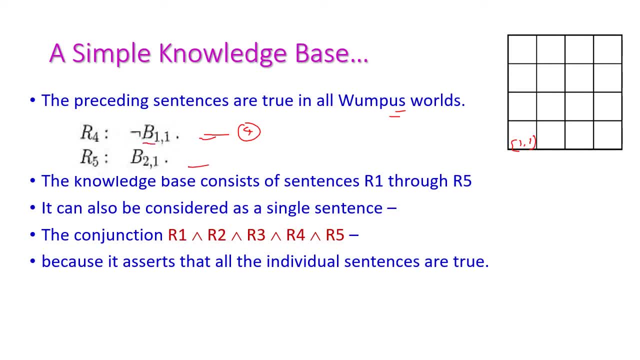 and breeze in 2 comma 1. breeze may be here. this is 2 comma 1, so these two sentences are always true, right, okay, here this is 5. the knowledge base consists of the sentences r1 through r5, so up to this we have 5 sentences of our knowledge base. right, and it can also be considered as a single. 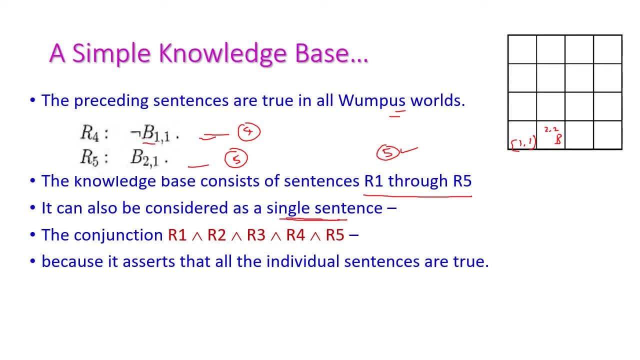 sentences, how we consider all these with single sentences. if all the sentences are true, then the final single sentence is true. if all the sentences are true, then the final single sentence, sentence that is, the conjunction of all those sentences, will also be true, Will also be true. 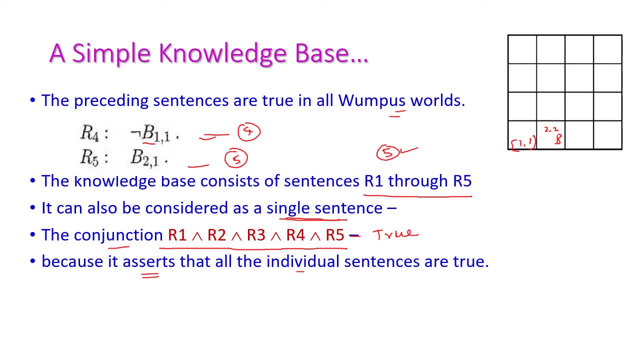 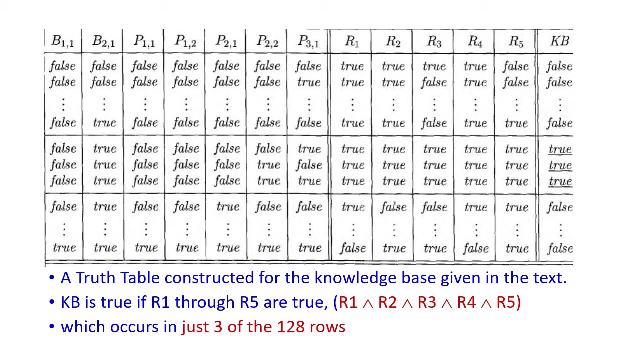 because it asserts that all individual sentences are true. All individual sentences are true, Okay. Next, with all these sentences, we try to construct a truth table. Okay, In this truth table, we are having all the possible variables sentences, Okay, So. 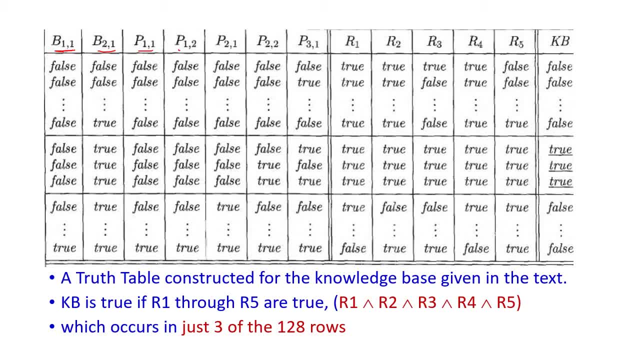 BF1,1,, BF1,2,, PF1,1,, PF1,2,, PF2,1,, PF2,2, PF3,1.. So after that we are having five sentences, isn't it? R1, R2, R3,, R4 and R5.. So with these things we try to give 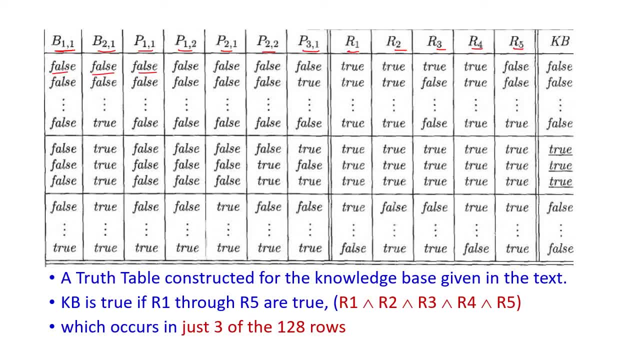 all possible combinations of true and false value for all these things. Okay, So, 1,, 2,, 3,, 4,, 5,, 6,, 7,, 8,, 9,, 10,, 11,, 12.. So, totally, 12 columns will be there. Okay, So 12 columns. 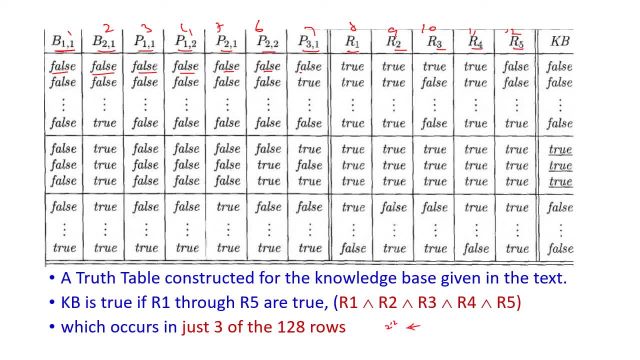 2 power: 12 possible rows will be there, So totally 128 rows will be Right. Okay, With all these combination, just only these three rows will get true value in the knowledge base. When the knowledge base will be true. if all the rows will be true, then the 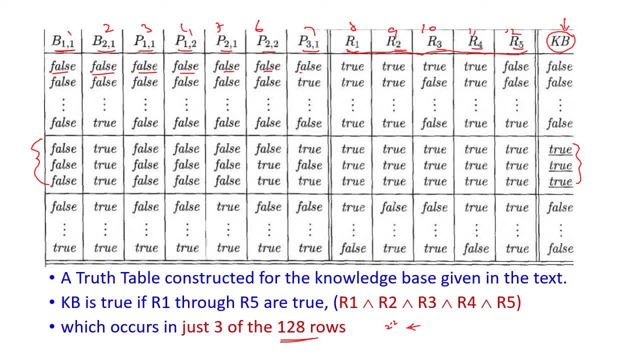 knowledge base will be true, Isn't it? Because we are doing the conjunction of all the rows? Isn't it? Conjunction of all the rows? If all the rows are true, then the knowledge base will be true. If all the rows will be true, then the entire knowledge base will also be true. Otherwise, 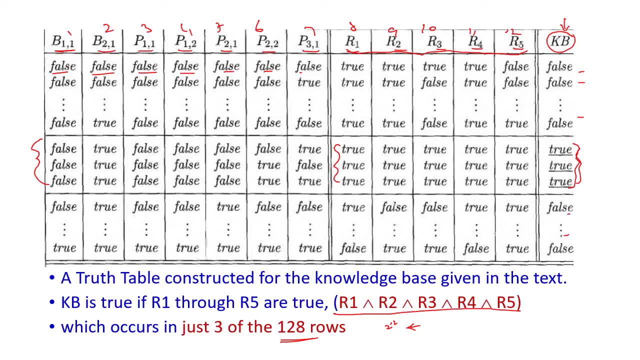 we will get only the false value, Only the false value. Okay, In what situation we will get this true value? B1, 1 always false and B2, 1 always be true and P of 1, 1 always false and P of 1, 2. 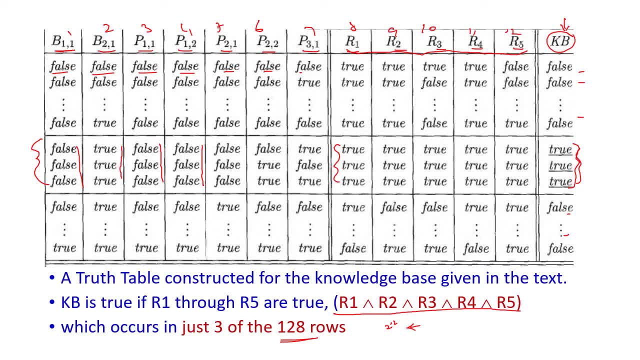 will always false, And P of 1, sorry, 2, 1 is also always false. Okay, If all these things are equal, then we will get true value in this knowledge base. Okay, Do you understand now? Okay, And only these two things will be changed. 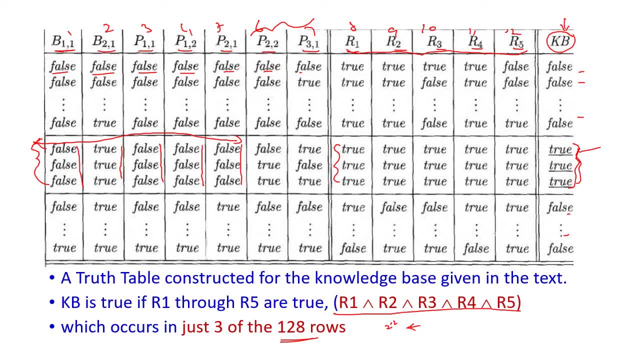 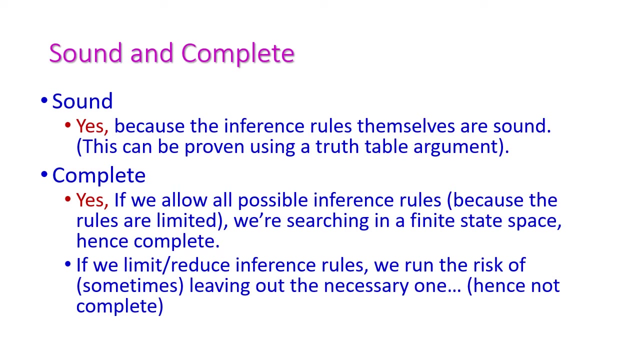 Okay, So this knowledge base value will highly depend on on these five variables. okay, so, among 128 rows, just three will be true in our knowledge base. and next let us see the sound and completeness of our example, that is, our knowledge base, by, with respect to our truth, table in this: 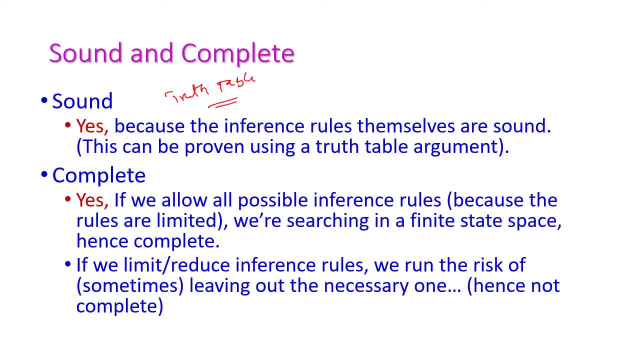 example: okay, vamper's world exam. first, soundness: in this example the soundness is S because the inference rule themselves are sound. all the inference rules will be true at one stage. okay, so in our truth table we are having Douglas, neuroscientist finding and tricks solving and alchemy. an example of close world consulting on focus might have lines to 절�ification of predicates in algo. so we write sekund Salman thesis. 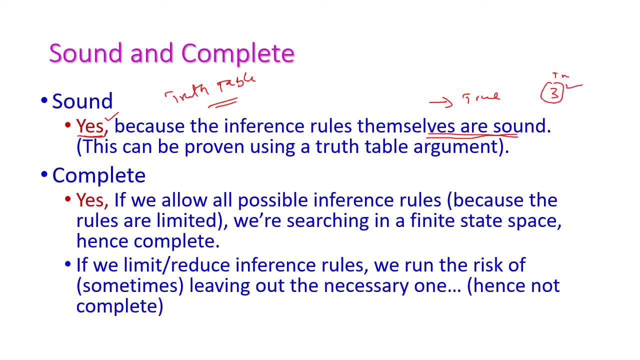 three possible true values in the knowledge base. isn't it the last column of our knowledge base? and this is proven by using our truth table argument. right, so it is a sound one. and next one is complete one, complete, yes, it is complete one because we allow the possible inference rule.